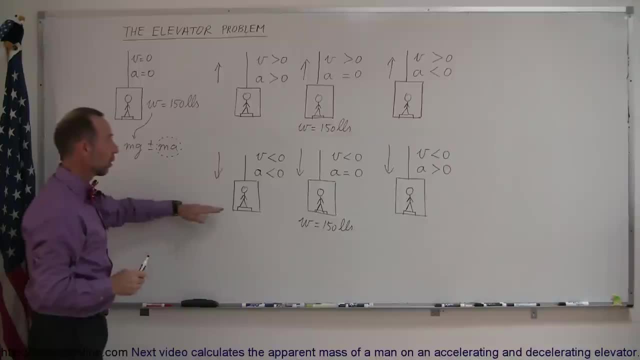 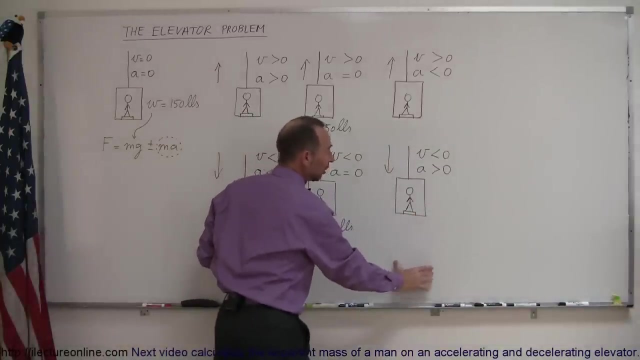 the elevator is slowing down and coming to its final destination. over here the elevators are moving downward, constant speed, here, here, from a standing position to a moving position. so excel accelerating downward, which is negative acceleration. and here the elevator is coming to its destination. it's slowing down, meaning if there's a positive acceleration, because it's 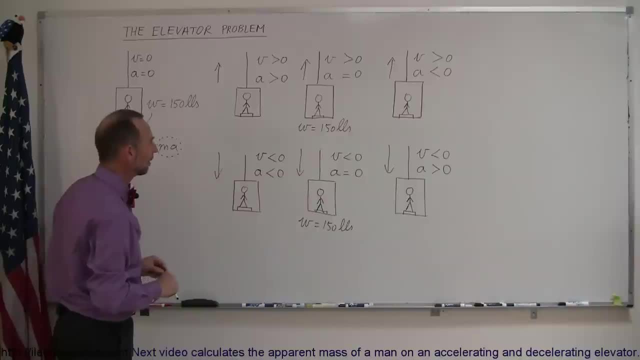 moving in a negative direction. so what would be the weight that the scale shows? well, in this case it would be: the weight is equal to the mg plus the ma. you would appear to be heavier because not only does the scale have to hold your weight up against gravity, it also. 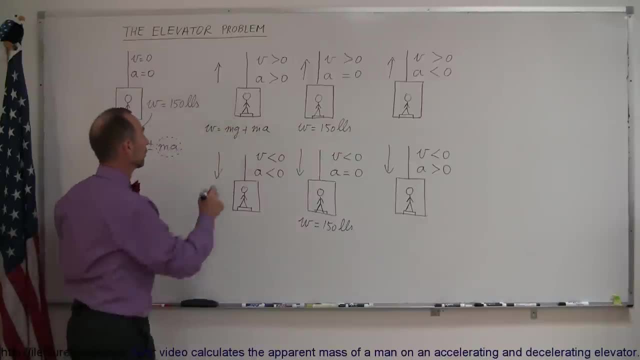 to push you upward at the acceleration a, and so therefore this would be equal to 150 pounds plus the ratio of a over g times 150 pounds. in other words, if the acceleration of the elevator is as much as g, which would be quite an elevator, then the person would appear to weigh 300 pounds. 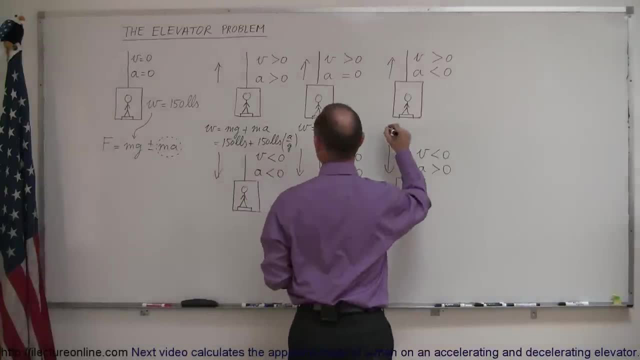 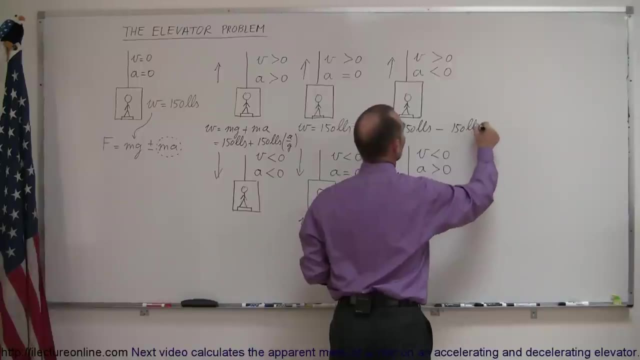 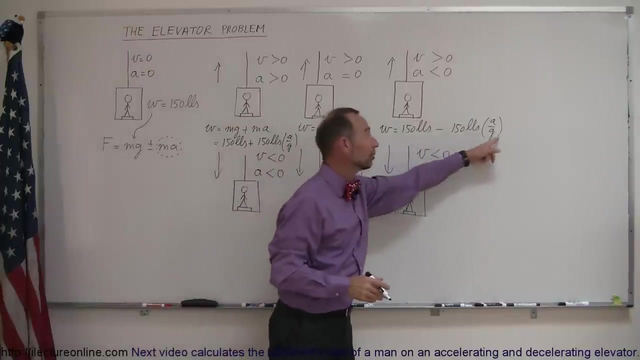 conversely over here, when the elevator is slowing down, then the weight here would be equal to 150 pounds, minus 150 pounds times the ratio of a over g. again, let's say that the elevator can slow down so quickly that a is equal to g, which is in minus 9.8 meters per second square, or minus 32 feet per. 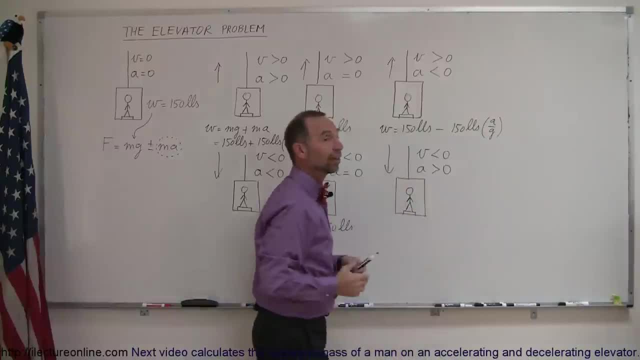 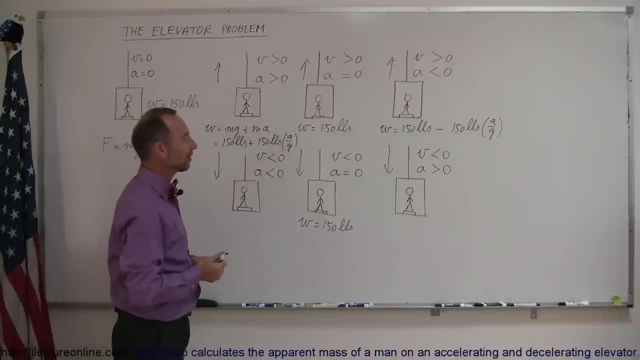 second square. then the person would temporarily be weightless as the elevator slows down. so usually elevators don't slow that down that fast because you know it would be quite a sensation to feel weightless at that moment. but that's how you would do that over here. 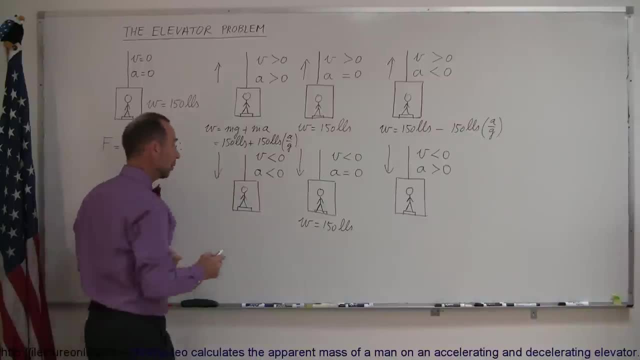 when the elevator is accelerating downward. for the moment you would feel like as if you're lighter. so the weight here is equal to 150 pounds minus the person's weight times the ratio of a over g. let's say that a is 10 percent of g, then this would be 15 pounds and the person would feel 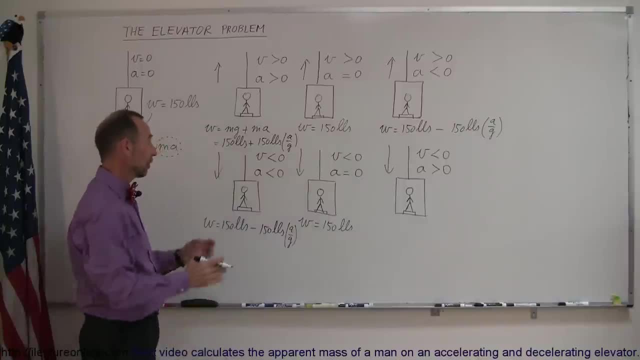 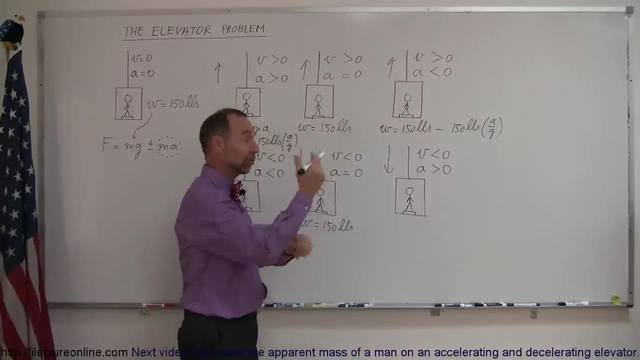 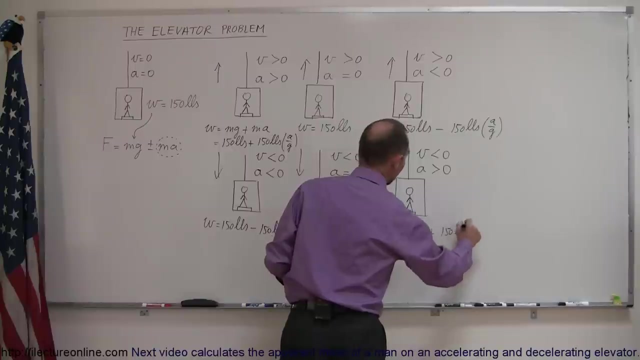 15 pounds lighter, as the elevator is beginning to move and so beginning to accelerate in a downward direction, but when the person reaches the final destination, the elevator is slowing with the acceleration upward. then we have: the weight is equal to 150 pounds plus 150 pounds.